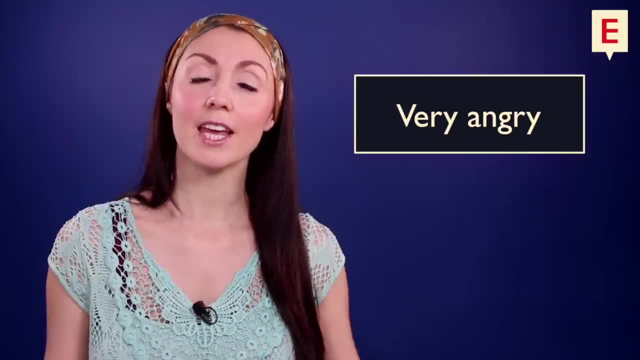 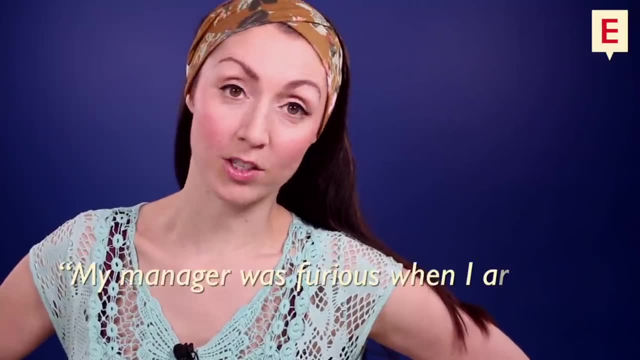 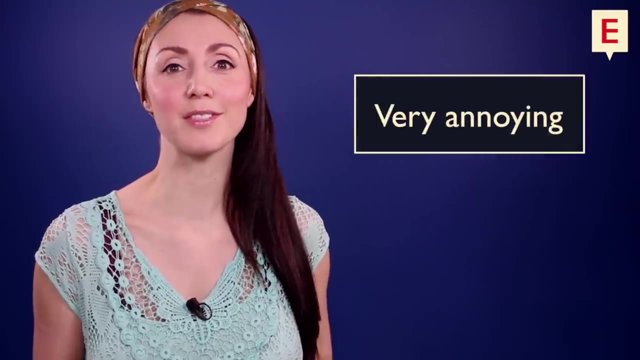 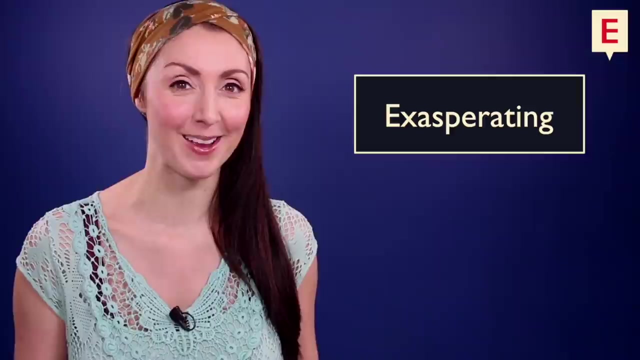 Ah. Number three: instead of saying very angry, try furious. My manager was furious when I arrived late for work this morning. Number four: instead of saying very annoying, try exasperating. Exasperating- To exasperate someone means to irritate them intensely. 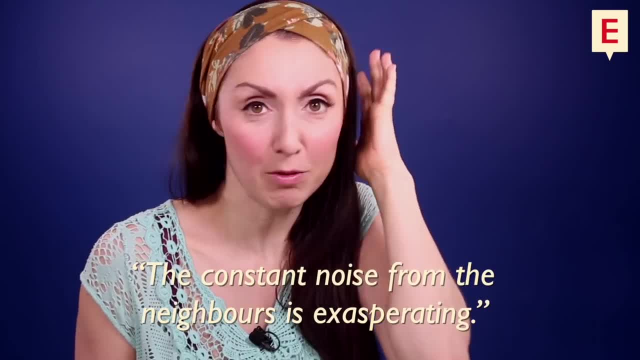 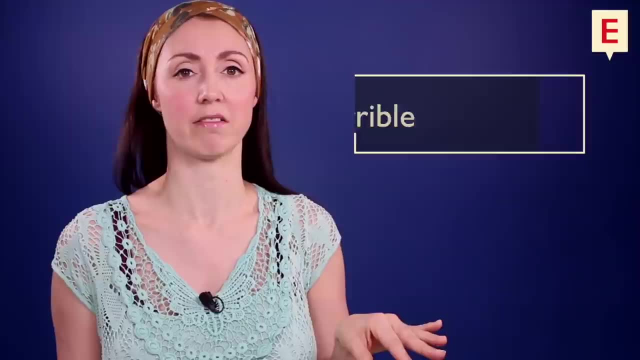 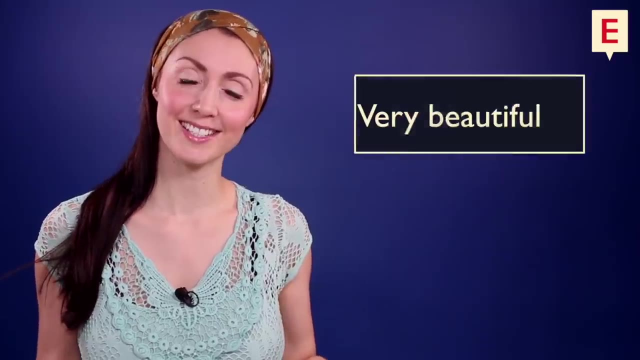 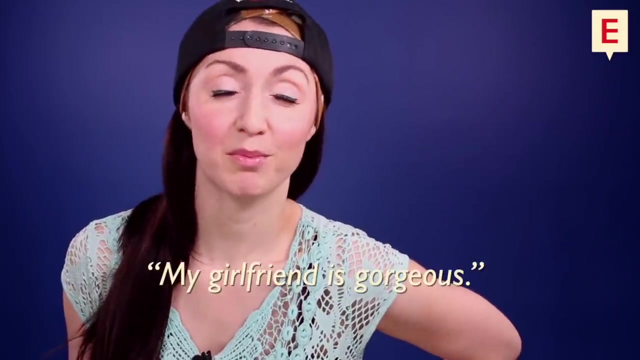 The constant noise from the neighbours is exasperating. Number five: instead of very bad, try terrible. I have a terrible headache. I may have to lie down. Number six: instead of very beautiful, try gorgeous. My girlfriend is gorgeous. 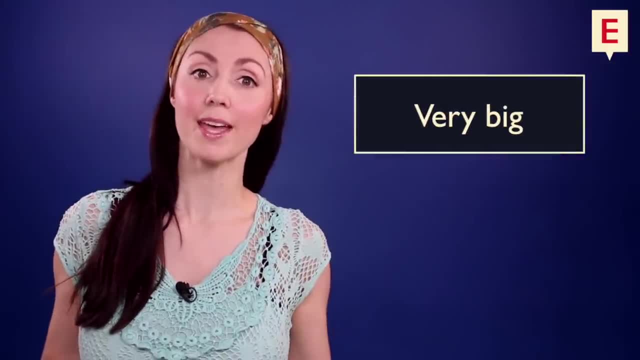 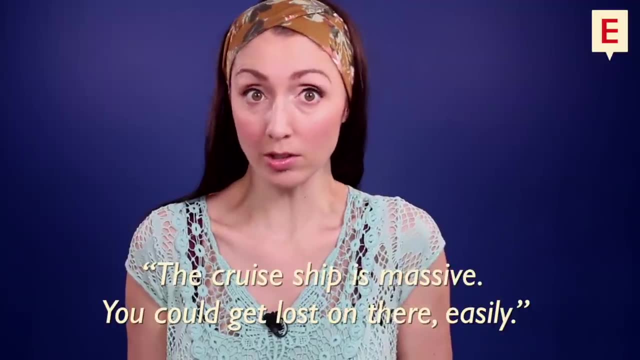 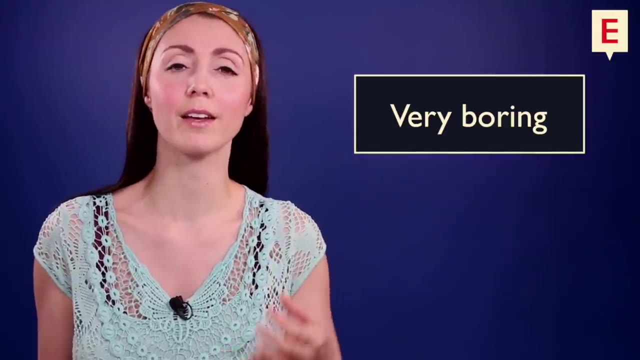 Number seven: instead of very beautiful, try gorgeous, My girlfriend is gorgeous. Number eight: instead of very big, try massive, The cruise ship is massive, You could get lost on there easily. Number eight: instead of saying very boring, try dull. Dull means lacking interest or excitement. 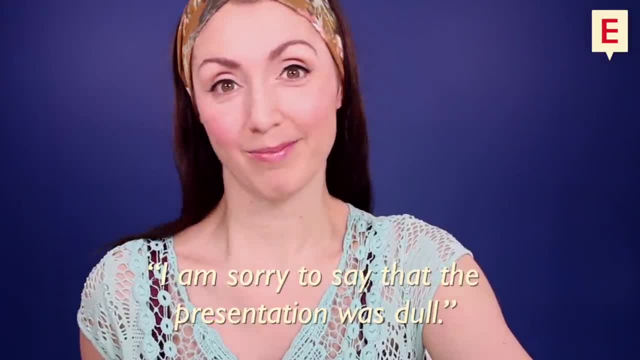 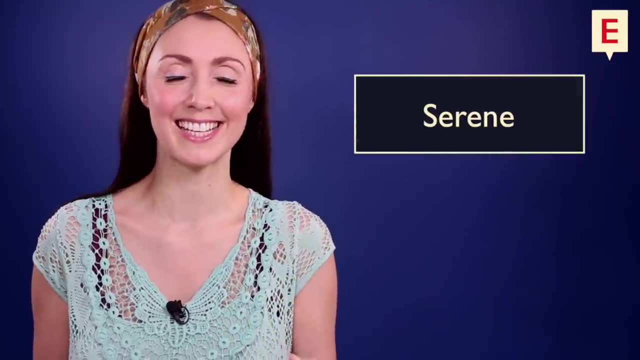 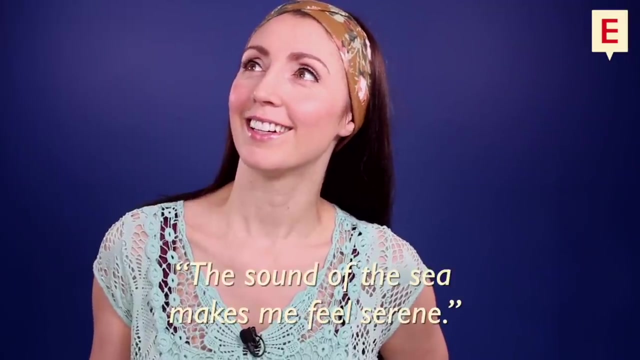 I'm sorry to say that the presentation was dull Number nine. instead of saying very calm, try dull, I feel serene, Serene. Sereane means calm, peaceful and untroubled. The sound of the sea makes me feel serene. 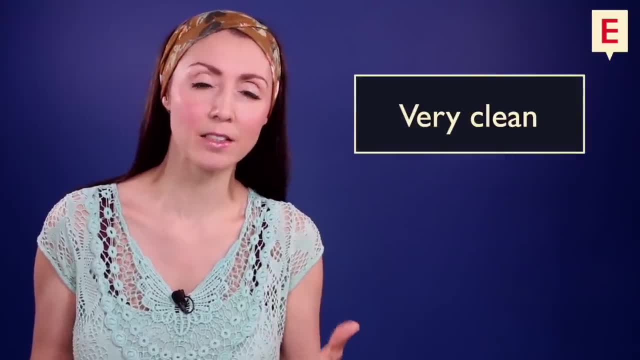 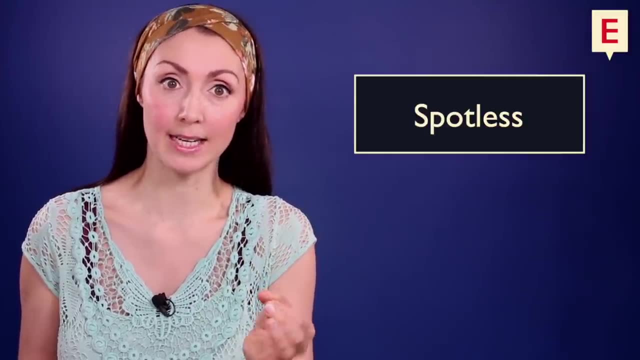 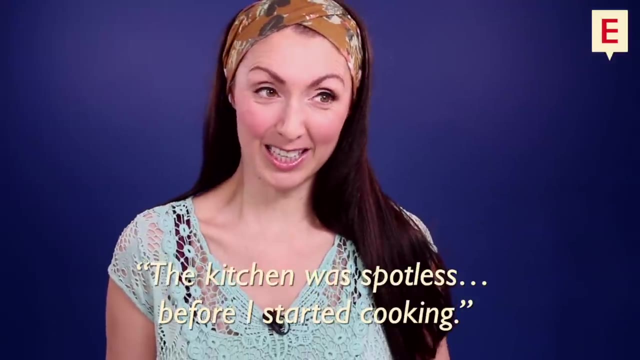 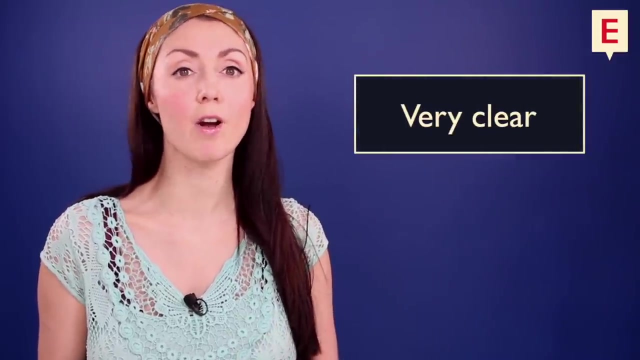 Number 10, instead of saying very clean, try spotless. If something is spotless, then it is immaculately clean without a spot. Uh, The kitchen was spotless before I started cooking. Number 11.. Instead of saying very clear, try obvious, obvious, obvious. 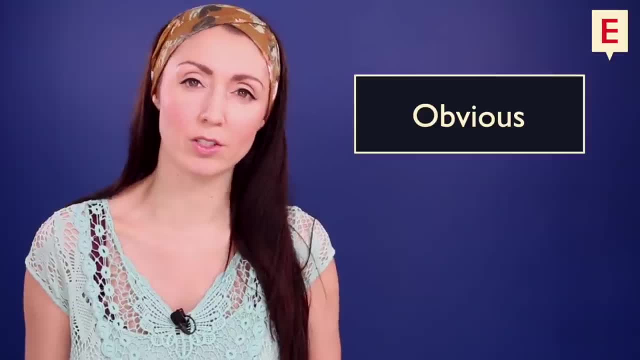 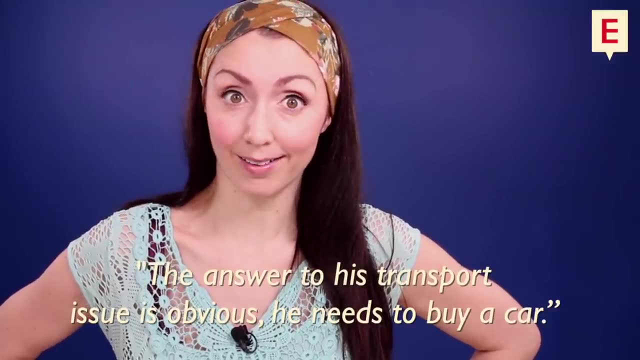 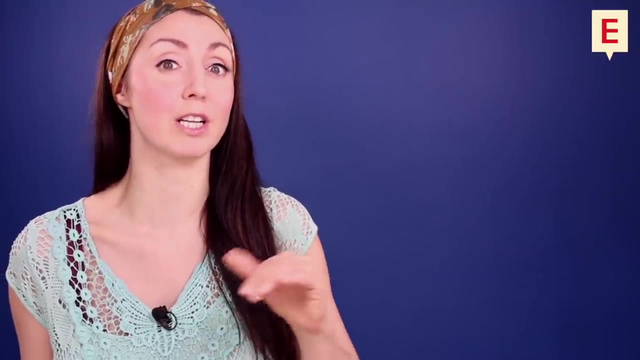 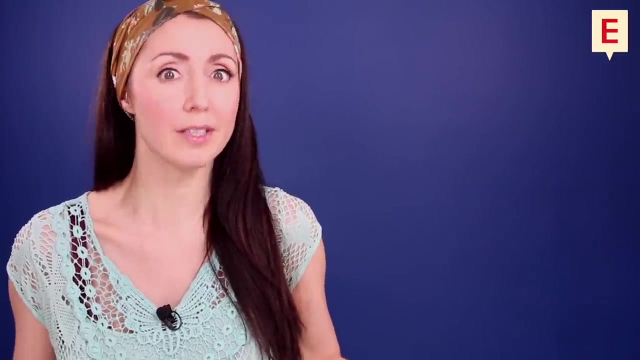 Obvious means easily perceived or understood. The answer to his transport issue is obvious: He needs to buy a car. One thing that is obvious is that studying intensely for three months will transform your language skills And getting 100% of your course fees back is obviously a wonderful incentive to work hard. 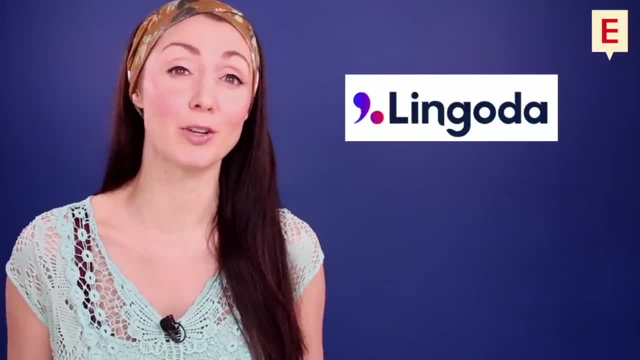 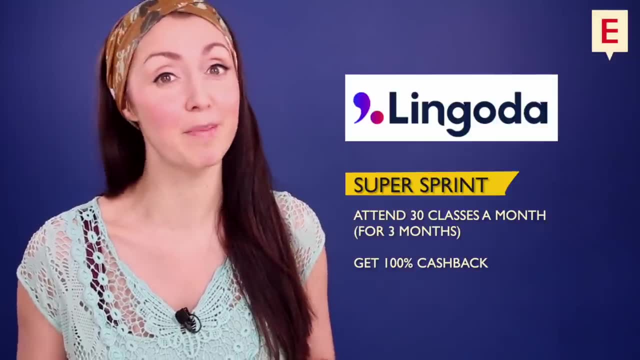 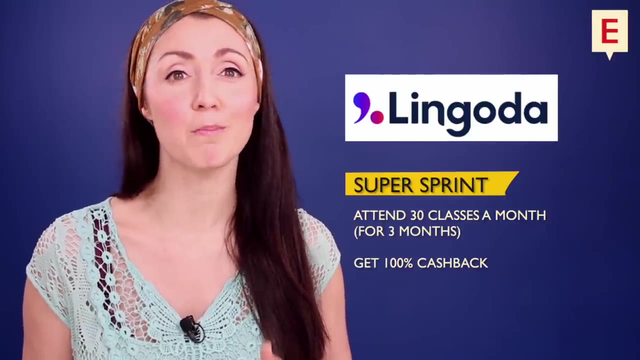 Now today's sponsor, Lingoda, are offering this opportunity. Sign up for their Super Sprint, which starts on the 2nd of August, Attend 30 classes a month for three months and get 100% Cash back. Amazing, This early bird offer is only available for a short time, so you must sign up before the 24th of June. 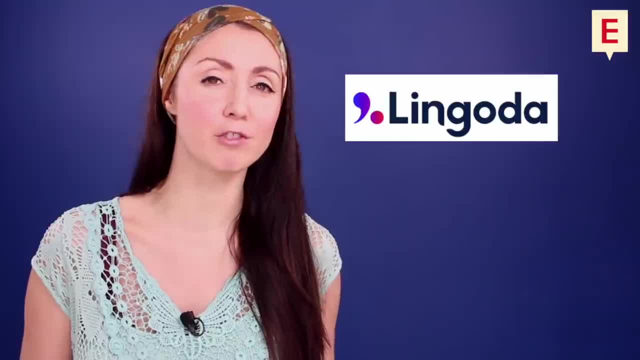 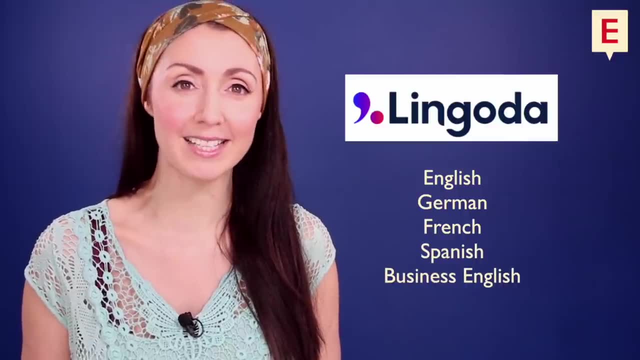 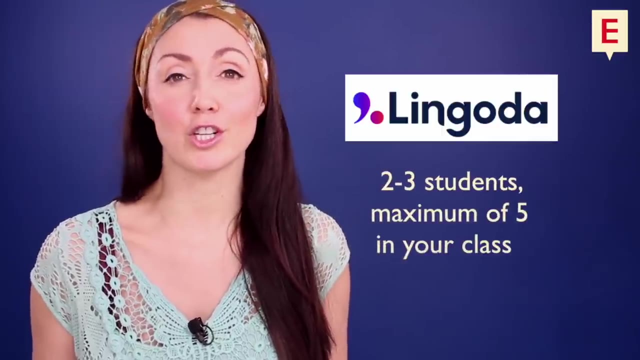 After which the cash back offer will come down from 100% to 50%. Languages you can learn are English, German, French, Spanish and Business English, And the interactive classes are run through Zoom and last for an hour. There are an average of two to three students, a maximum of five in your class. 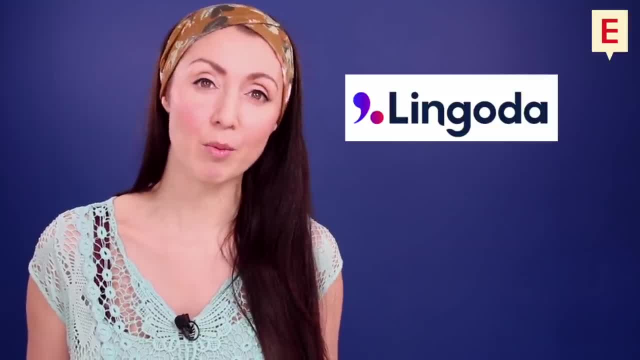 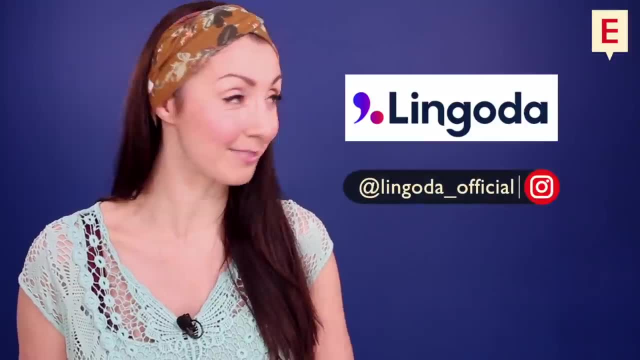 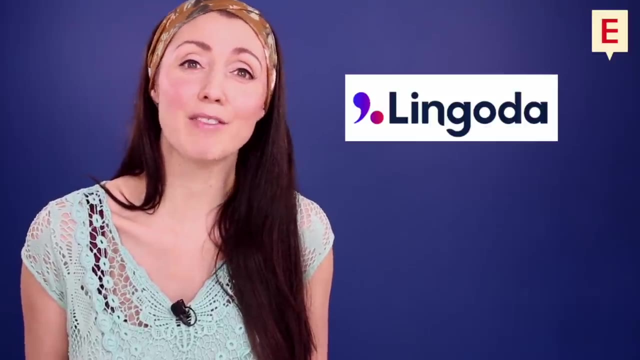 So the teacher has a great opportunity To interact with everyone and give you lots of feedback. You can check out what Lingoda students are saying on their Instagram story highlights Now. if a class every day for three months is too intense for you, then you have an option. 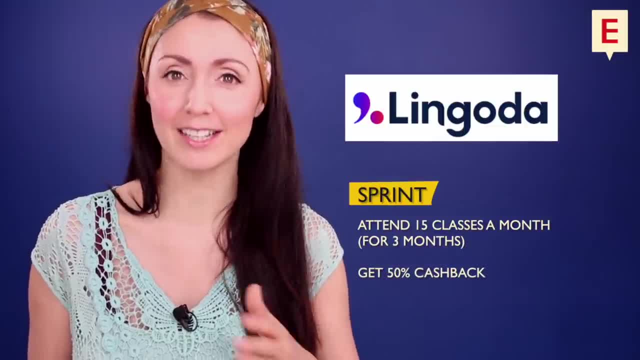 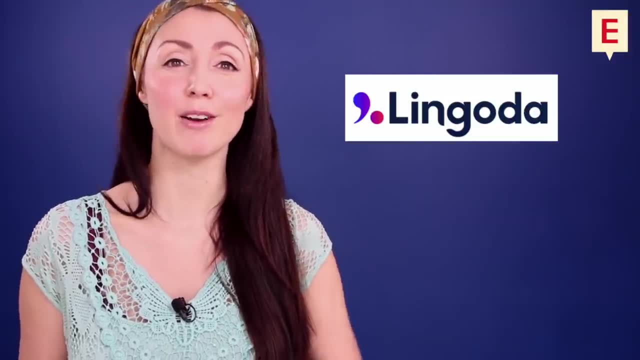 Join the Sprint. instead, You attend 15 classes a month for three months and get 50% cash back. Sign up with my link and use this voucher code To get a 20% cash back. 20 euro discount on the deposit. 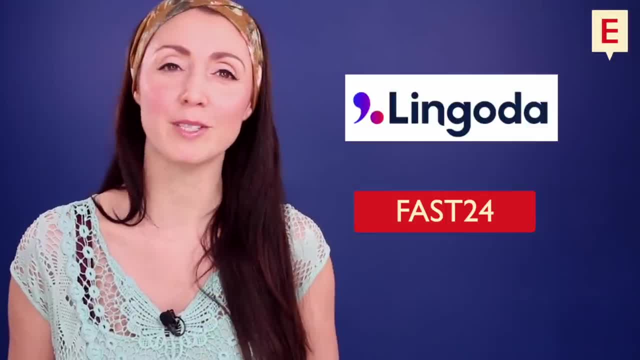 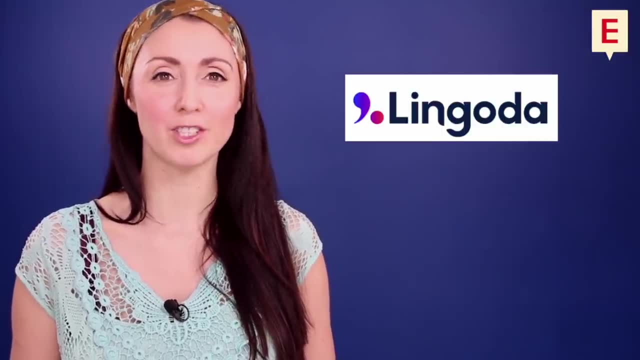 If you're aiming high, sign up for the Super Sprint with 100% cash back, but sign up before the 24th of June. Don't forget to check out their frequently asked questions section before signing up. Now back to the lesson. 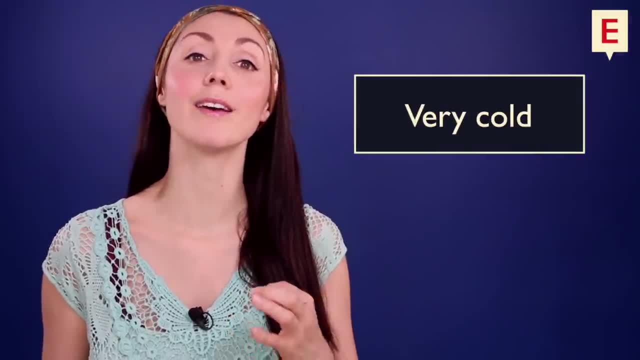 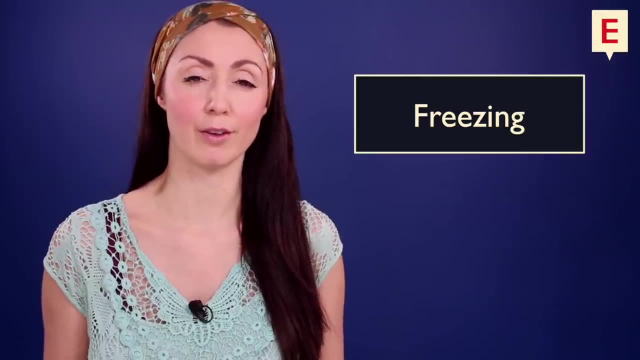 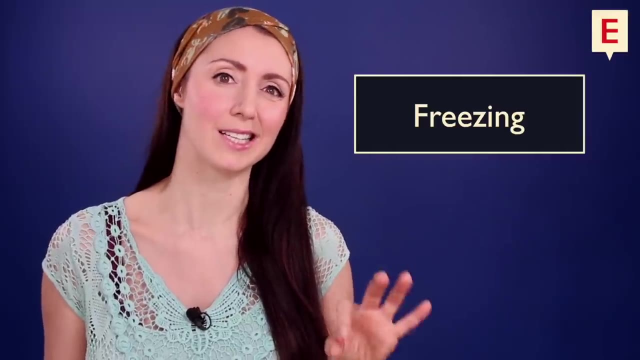 Number 12. Instead of saying very cold, try freezing. If something is freezing, it literally means it has reached a freezing temperature of below zero, but we colloquially use it As an adjective to mean extremely cold, even if it's not quite literally freezing. 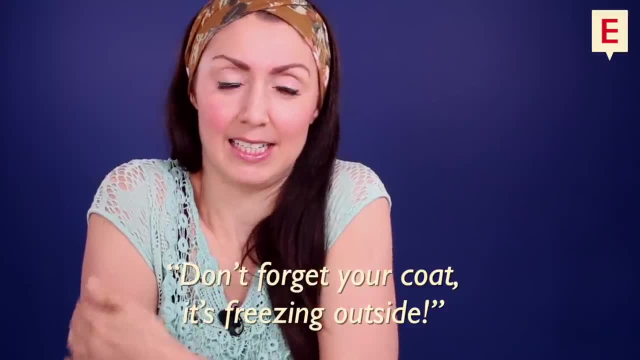 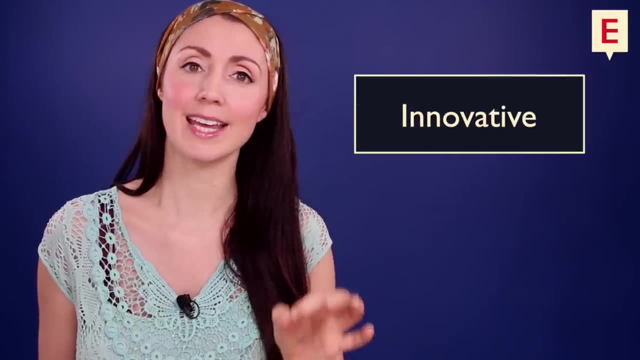 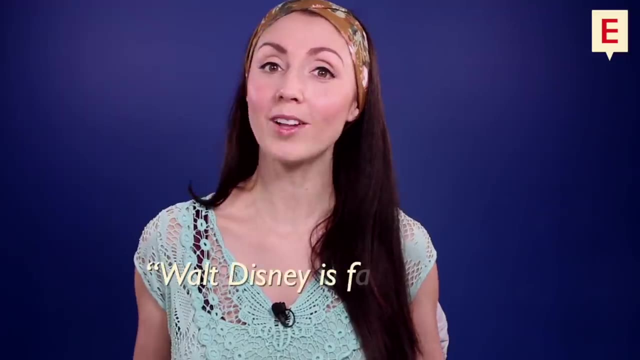 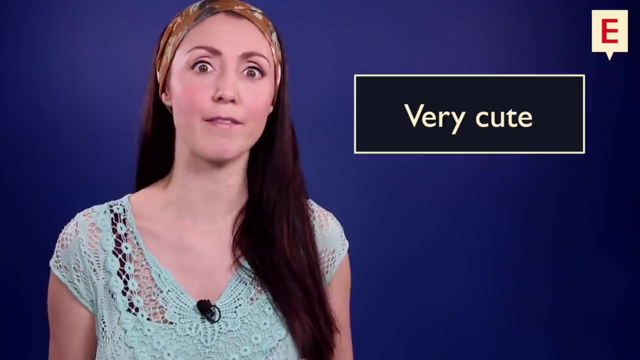 Don't forget your coat. It's freezing outside, Number 13.. Instead of saying very creative, try innovative, Innovative. Innovative means new, advanced and original. Walt Disney is famous for his innovative work In animation- Number 14.. Instead of saying very cute, try adorable. 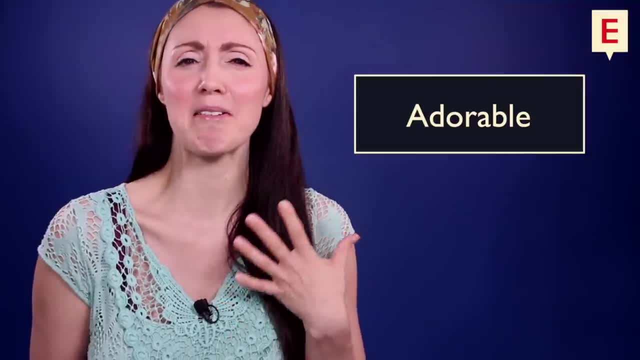 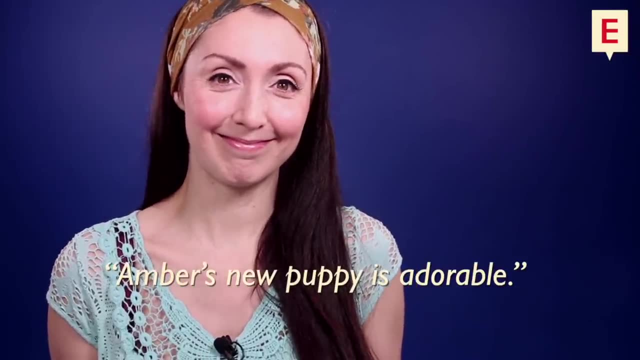 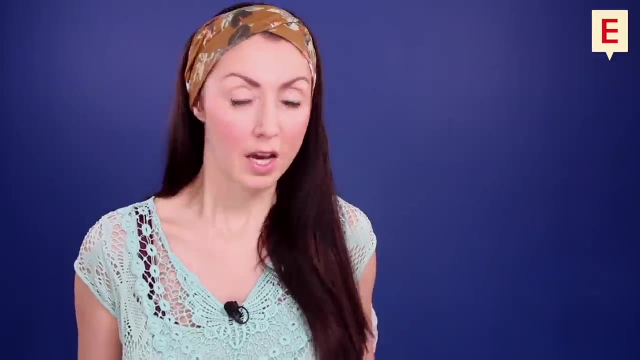 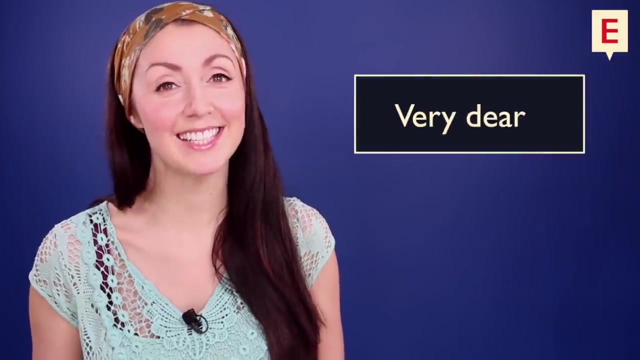 Adorable means inspiring great affection. Oh, Amber's new puppy is adorable, Number 15.. Instead of saying very dangerous, try perilous. The journey to the top of the mountain was perilous, Number 16.. Instead of saying very dear, try cherished. 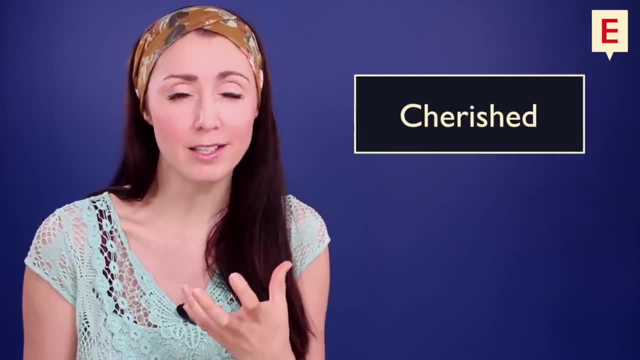 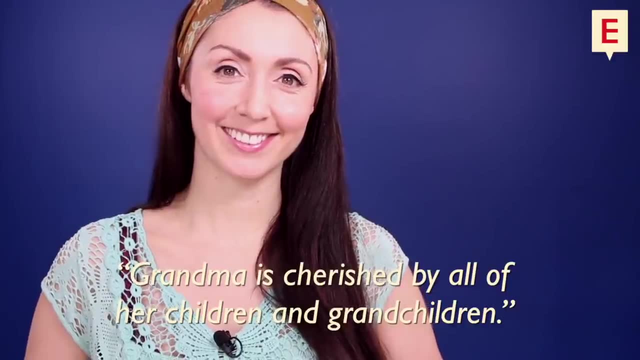 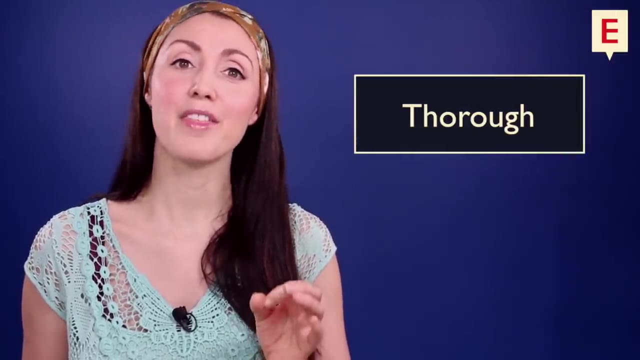 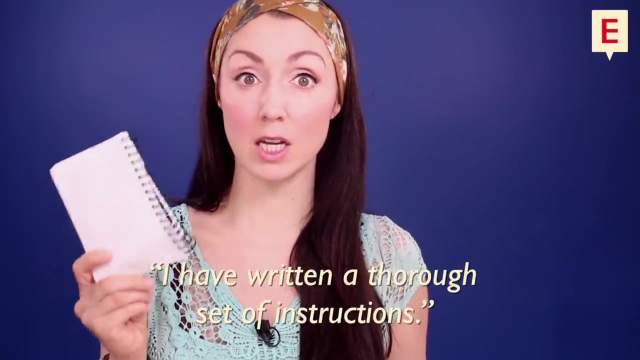 To cherish something means to protect and care for it lovingly. Grandma is cherished by all of her children and grandchildren- Number 17.. Instead of saying very detailed, try thorough. Thorough means completed carefully and meticulously Right. I've written a thorough set of instructions. 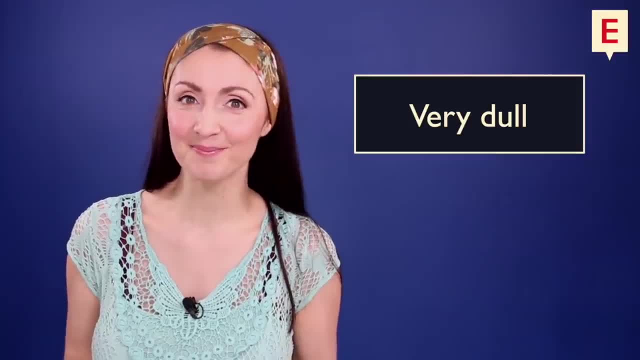 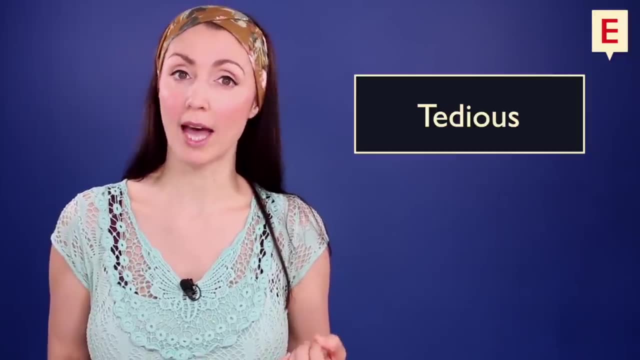 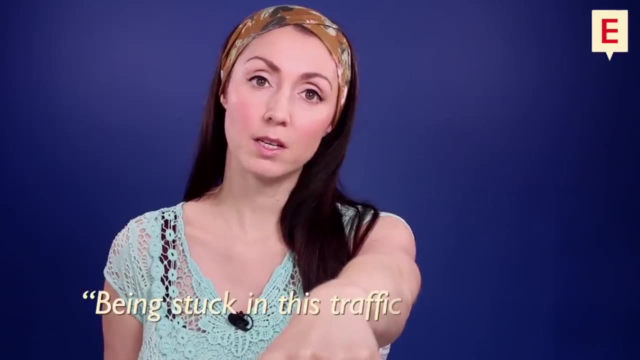 Number 18.. Instead of saying very dull, try tedious. If something is tedious, then it is long, slow and boring to an extent where it feels tiresome and monotonous. Being stuck in this traffic is tedious, Number 19.. 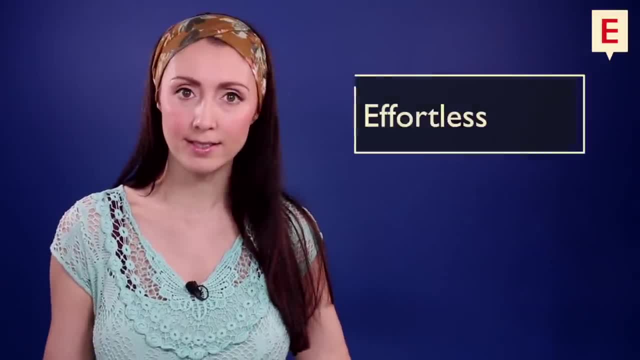 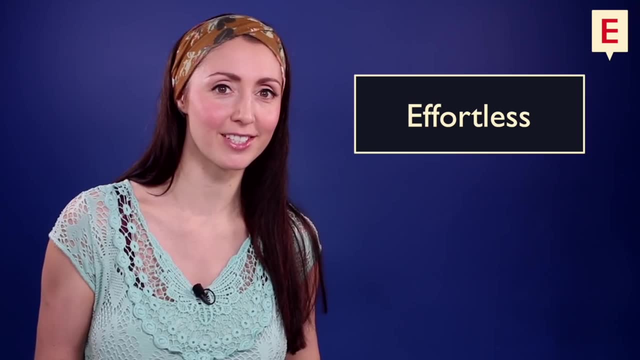 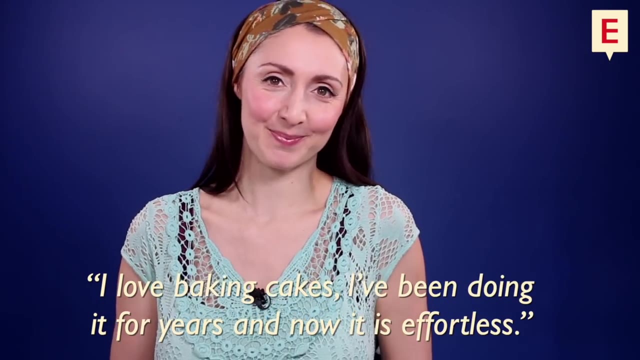 Instead of saying very easy, try effortless. If something is described as effortless, it is achieved with ease and without much effort. Oh, I love baking cakes. I've been doing it for years and now it's effortless Number 20.. Instead of saying very excited, try thrilled. 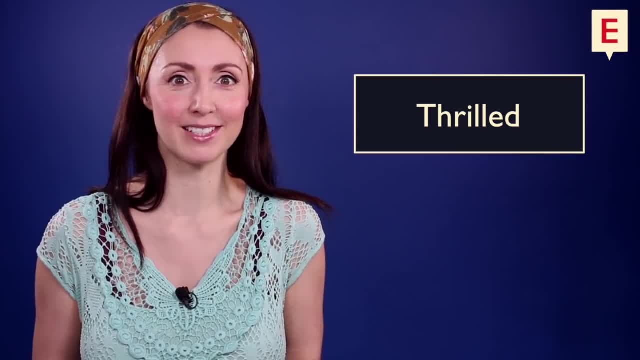 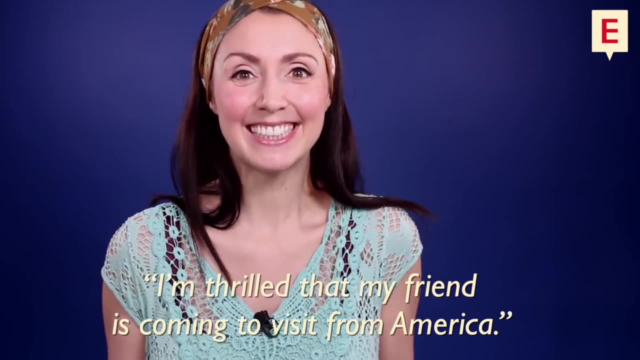 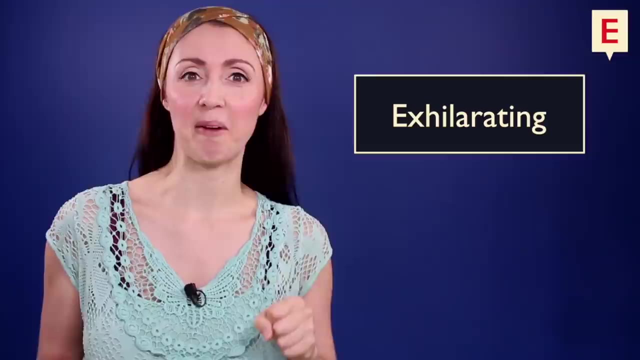 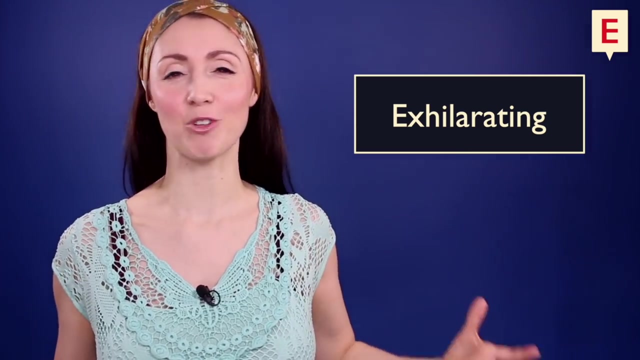 To be thrilled means to feel sudden excitement. Oh, I'm thrilled that my friend is coming to visit from America Number 21.. Instead of saying very exciting, try exhilarating. If something is exhilarating, it makes you feel happy, animated or excited. 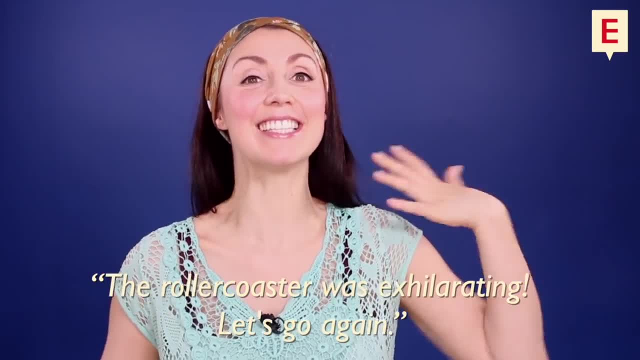 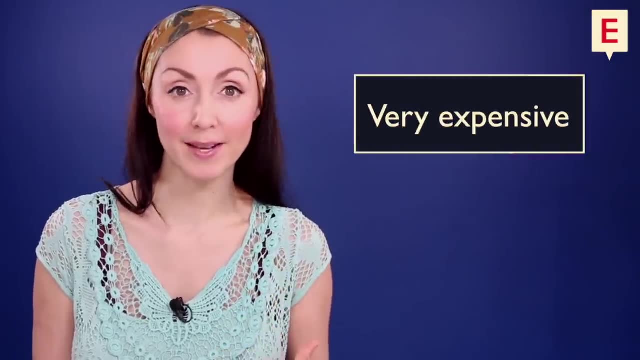 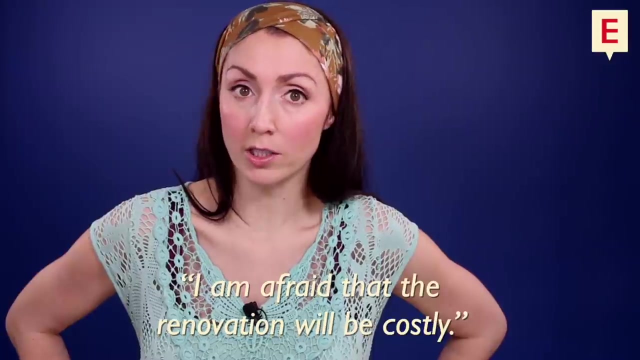 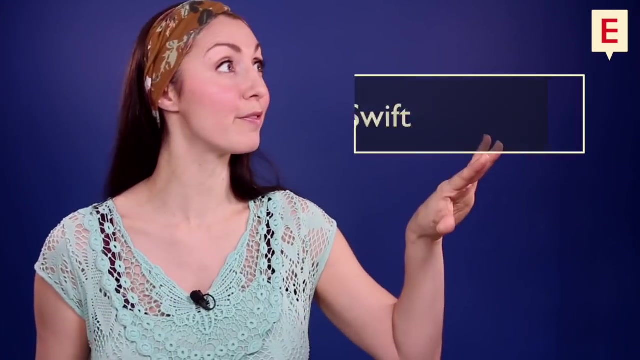 Whoa, the roller coaster was exhilarating. Let's go again. Number 22. Instead of saying very expensive, try costly. I'm afraid that the renovation will be costly. Number 23. Instead of saying very fast, try swift. 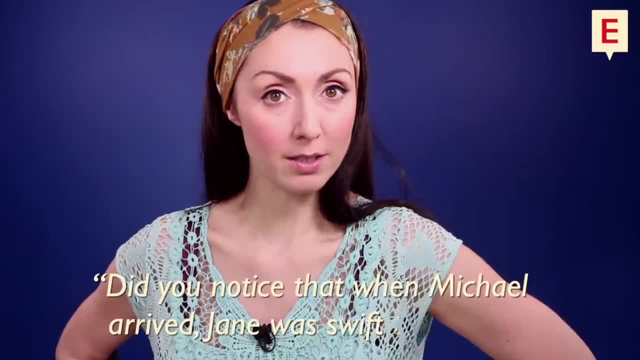 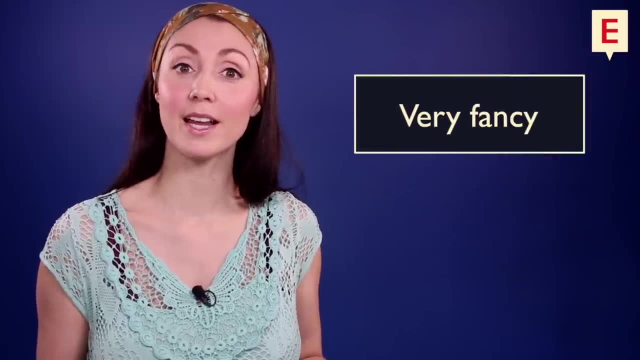 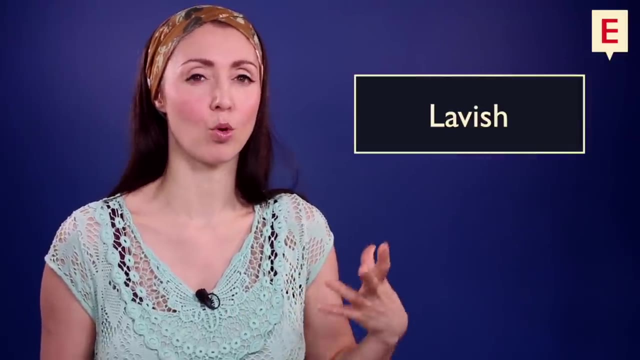 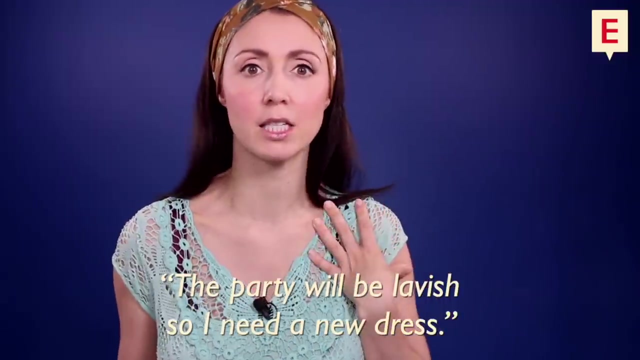 Swift means happening quickly. Did you notice that when Michael arrived, Jane was swift to leave Number 24.. Instead of very fancy, Try lavish. Lavish means rich, elaborate or luxurious. The party will be lavish. so I need a new dress. 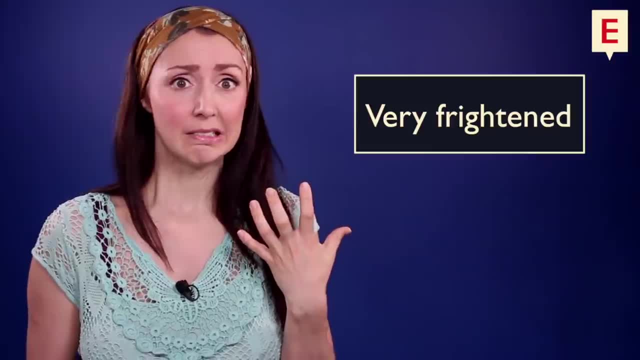 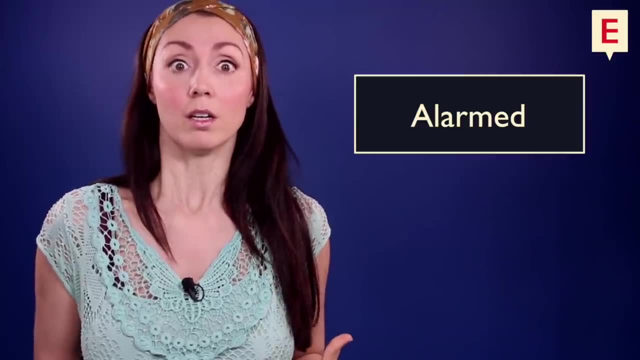 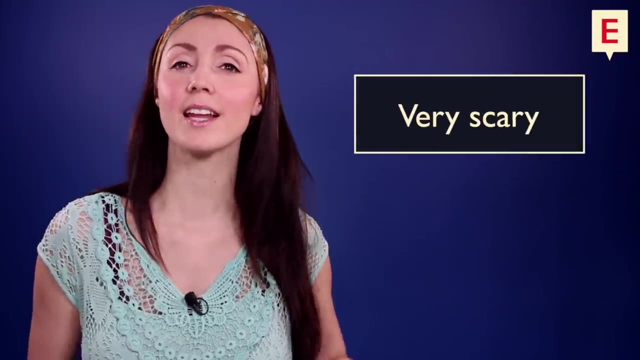 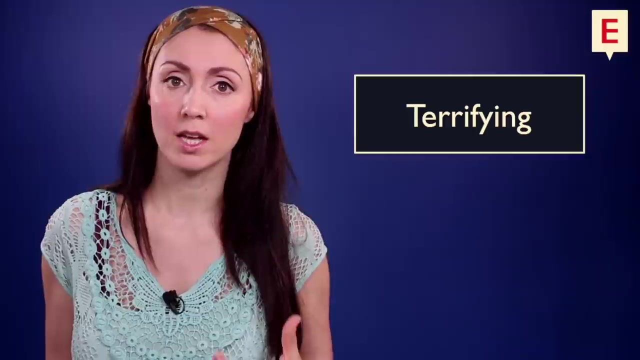 Number 25.. Instead of very frightened, try alarmed To be alarmed means to feel frightened or in danger. I was alarmed to find that the front door was open- Number 26.. Instead of very scary, try terrifying. If something is terrifying, it causes extreme fear. 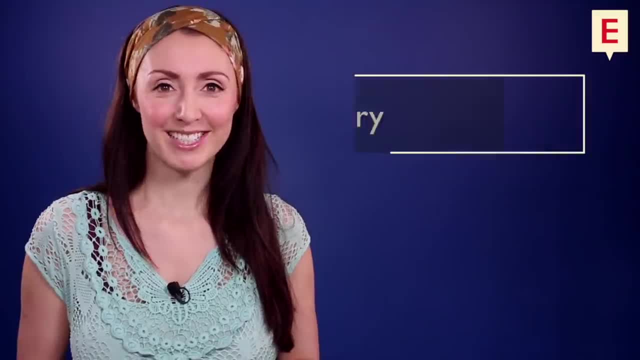 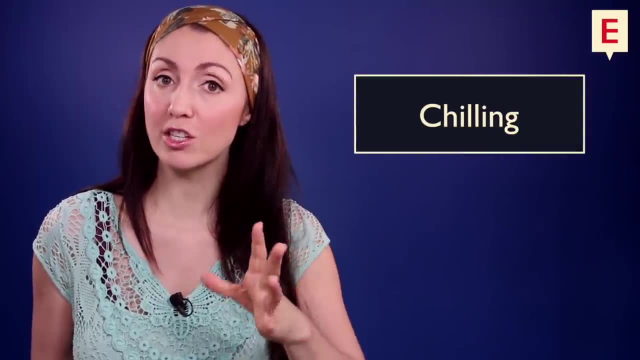 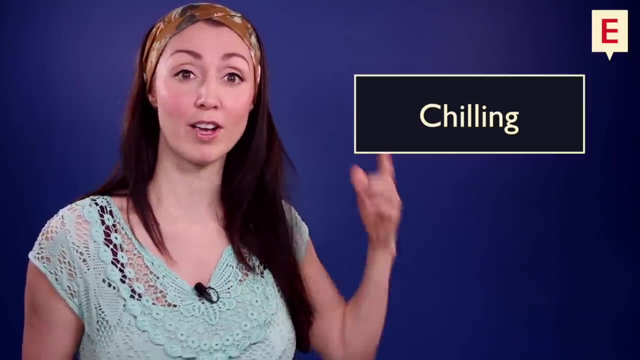 Horror movies are terrifying, Number 27.. Another alternative to very scary You could try chilling. If something is chilling, then it is horrifying or frightening to an extent where it makes you feel a chill Or a shiver down your spine. Tina told a chilling ghost story. 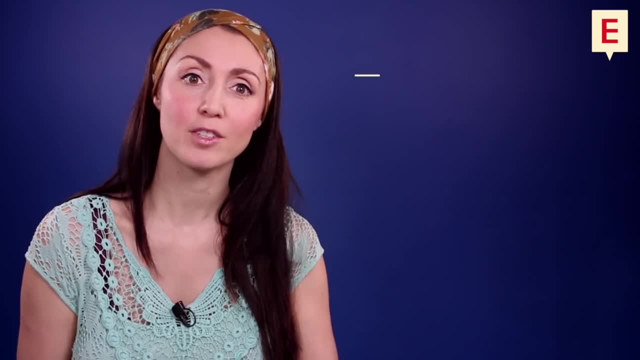 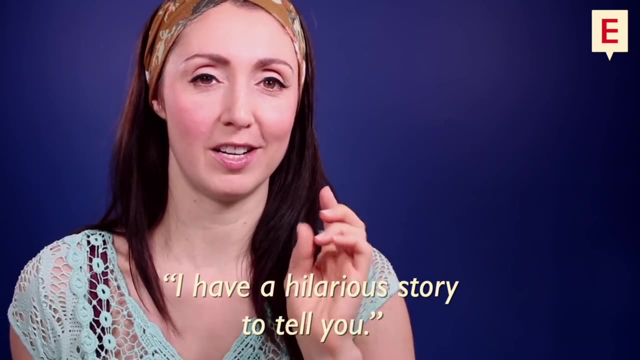 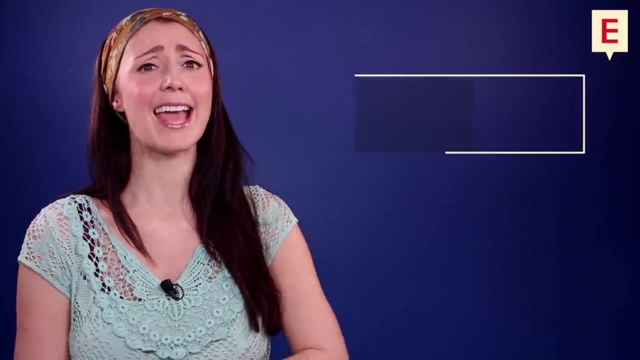 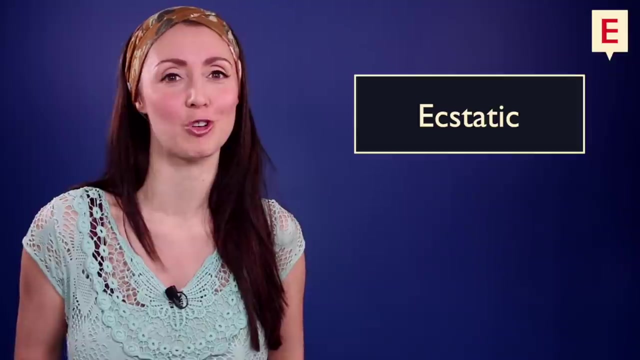 Number 28.. Instead of very funny, try hilarious. I have a hilarious story to tell you, Number 29.. Instead of very happy, try ecstatic. To be ecstatic means to feel ecstatic, To feel an overwhelming sense of happiness or joy. 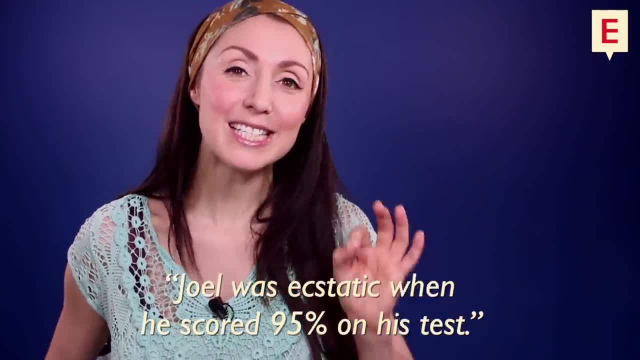 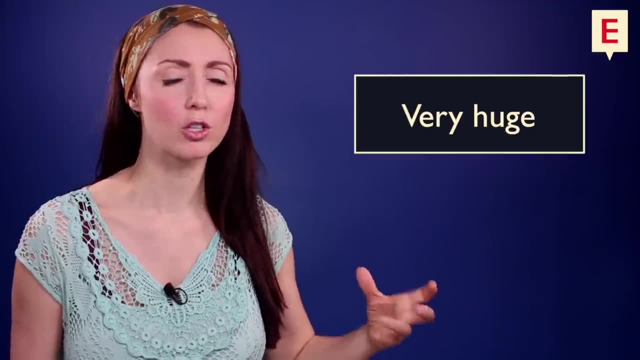 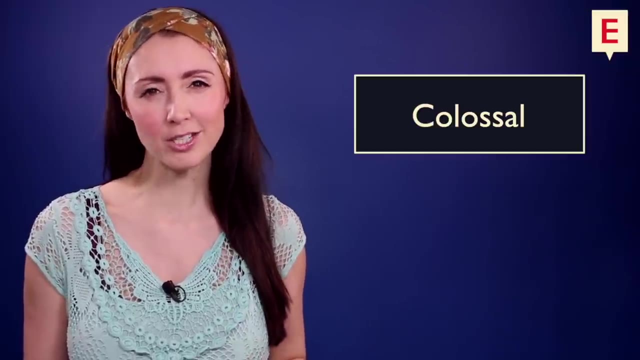 Joel was ecstatic when he scored 95% on his test Number 30.. Instead of very huge, try colossal. Now, because huge is already a non-gradable adjective, it's actually grammatically incorrect to use very as a modifier here. 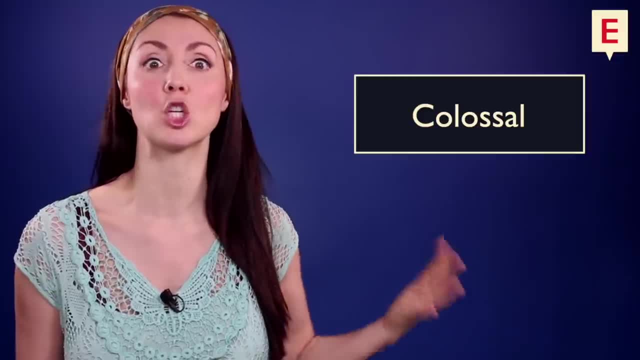 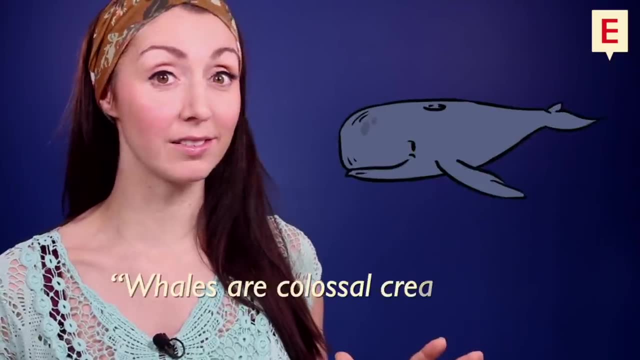 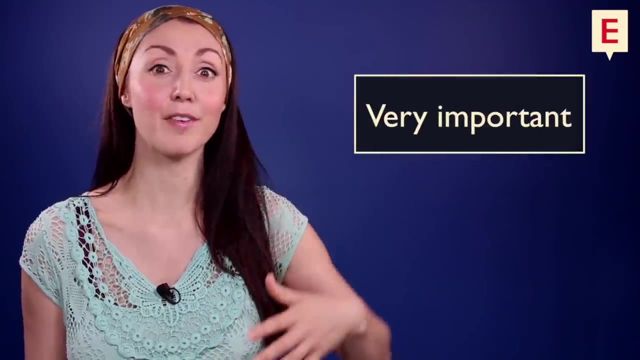 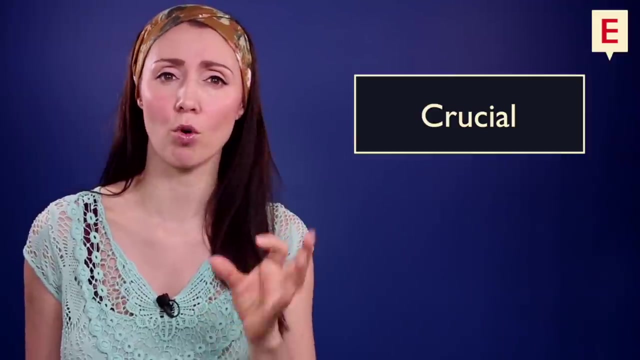 You could emphasize it by saying: something is absolutely huge, Or you could opt for another word altogether like colossal Whales are colossal creatures Number 31.. Instead of very important, try crucial. If something is crucial, then it is of great or critical importance. 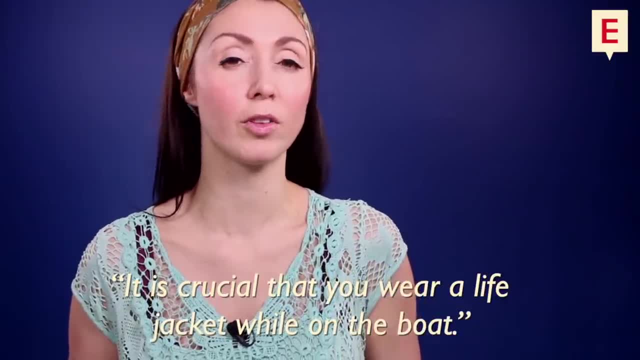 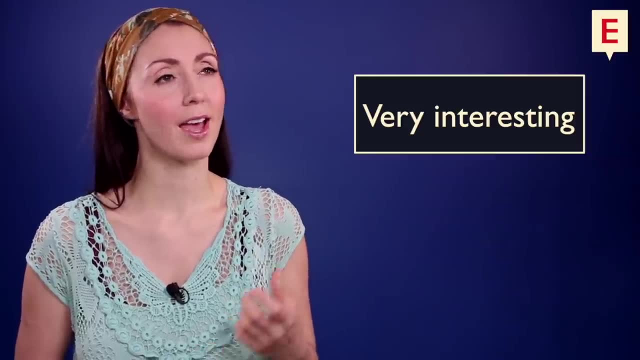 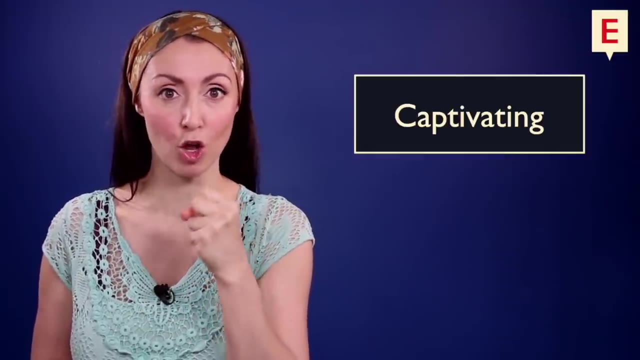 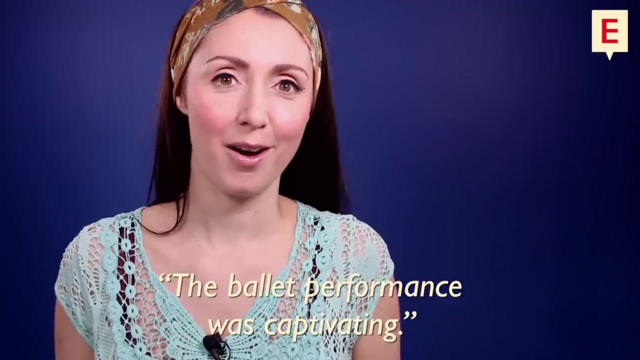 It is crucial that you wear a life jacket while on the boat, Number 32.. Instead of very interesting, try captivating. If something is captivating, it attracts and holds your attention for a long time. The ballet performance was captivating- Number 33.. 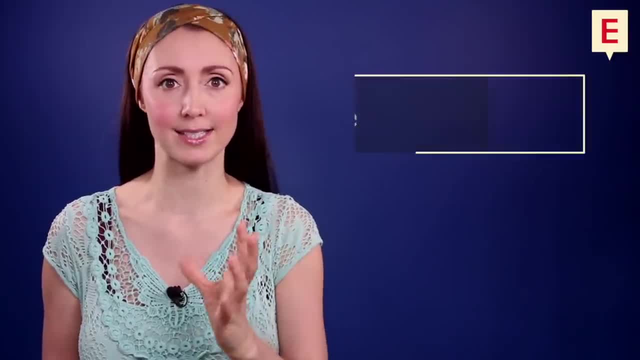 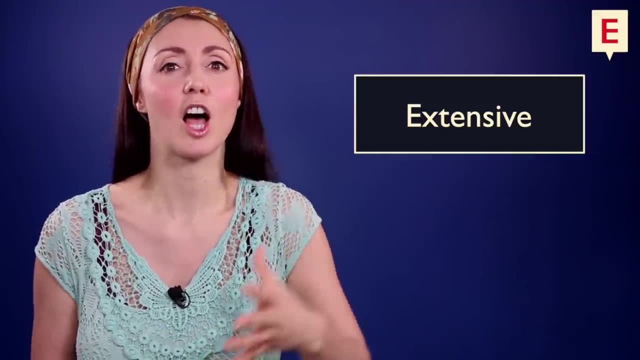 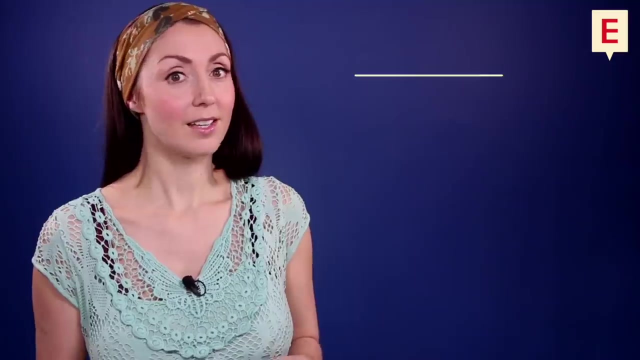 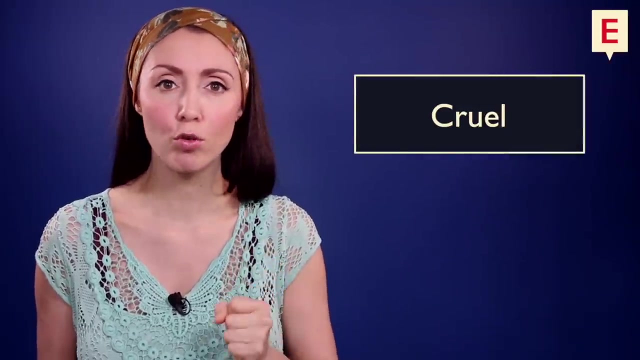 Instead of very long, try extensive. Extensive means covering or affecting a large area or, in this case, a long time. Becoming fluent in English is an extensive process. Number 34. Instead of very mean, try cruel To be. cruel means to intentionally cause pain or suffering without feeling concern. 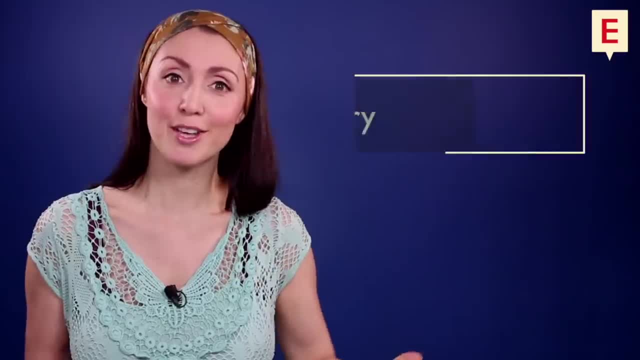 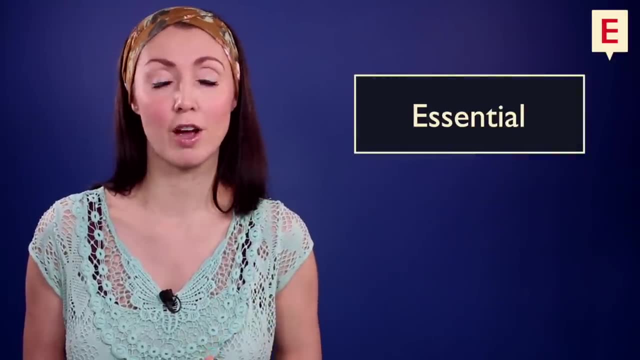 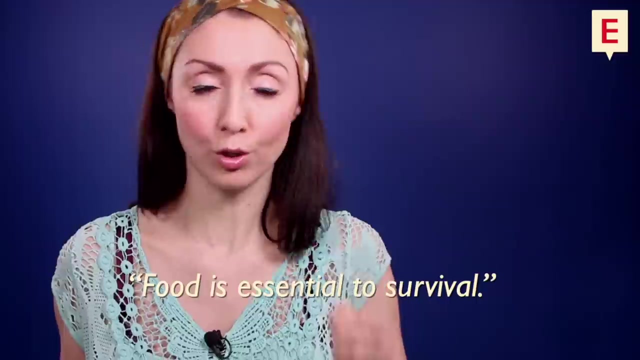 School bullies can be cruel. Number 35.. Instead of very necessary, try essential. Now, if something is described as essential, then it is extremely important and you can't be without it. Food is essential to survival- Number 36.. 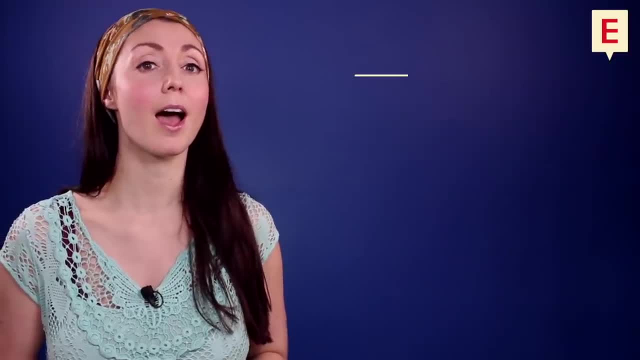 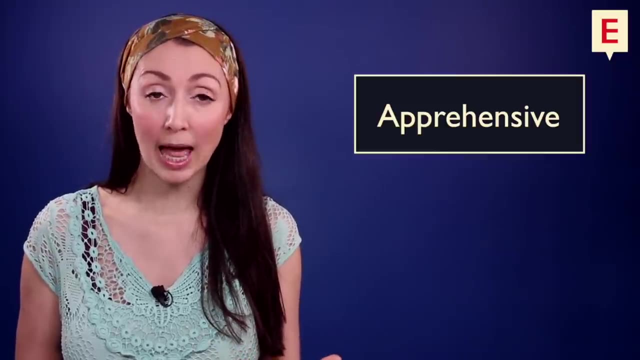 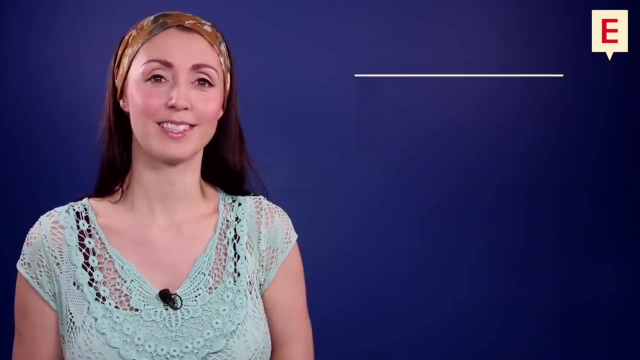 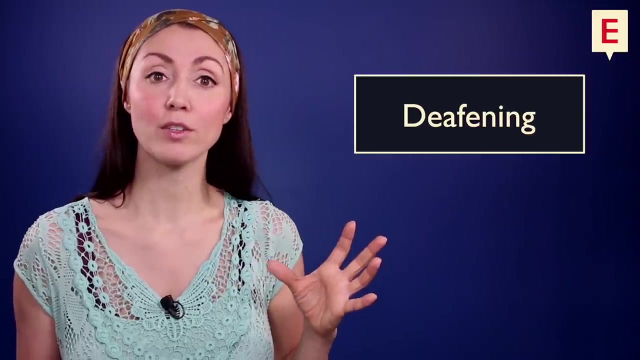 Instead of very nervous, try apprehensive. To be apprehensive means to feel anxious or worried that something bad will happen. Kyle is apprehensive about moving schools. Number 37.. Instead of very noisy, try deafening. If a noise is deafening, it is so loud that it is impossible to hear anything else. 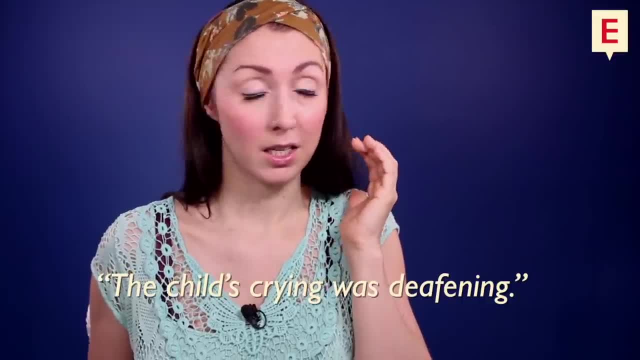 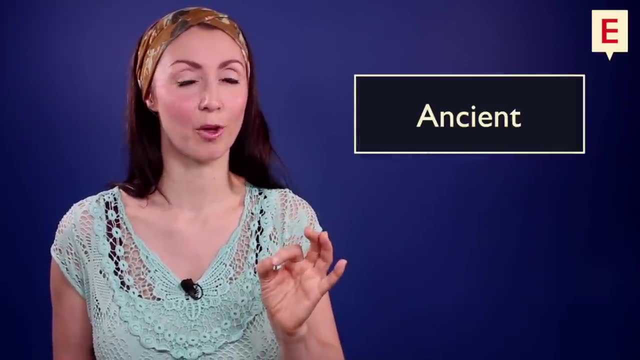 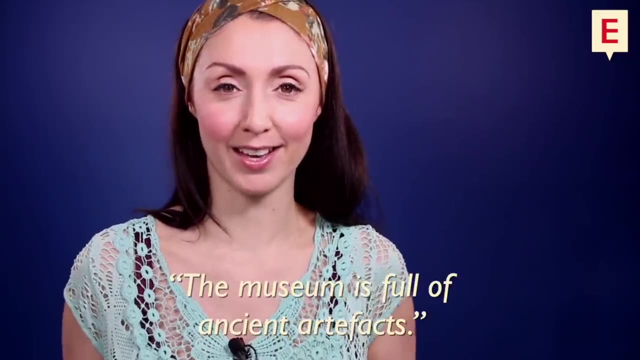 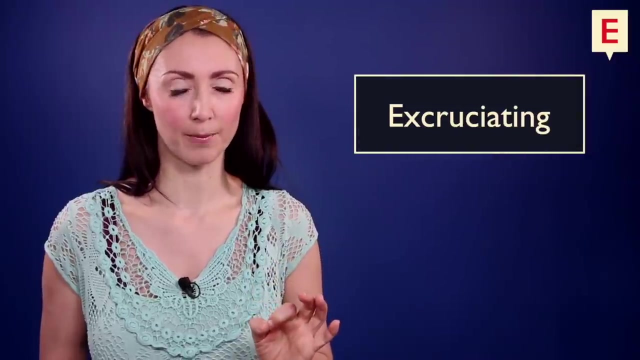 The child's crying was deafening. Number 38. Instead of very old, try ancient. Ancient means belonging to the very distant past. The museum is full of ancient artefacts. Number 39. Instead of very painful, try excruciating. 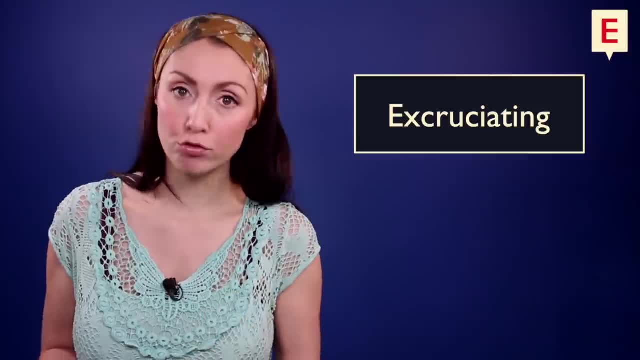 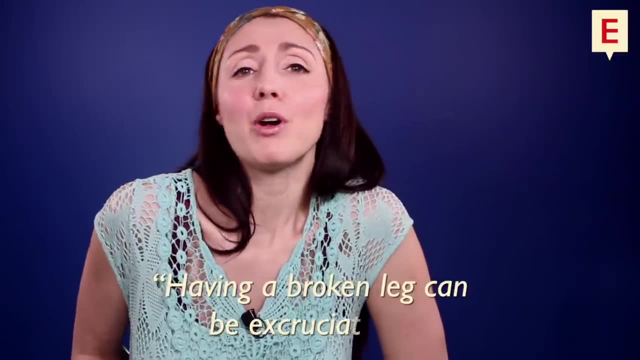 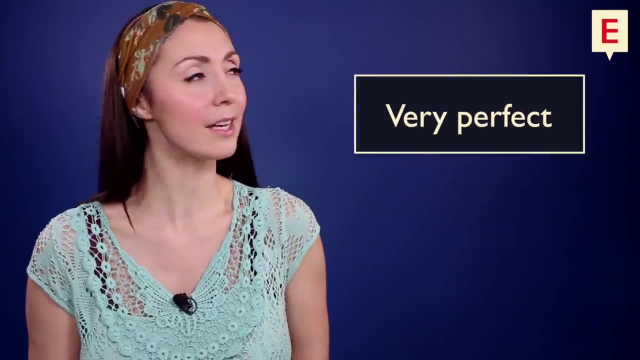 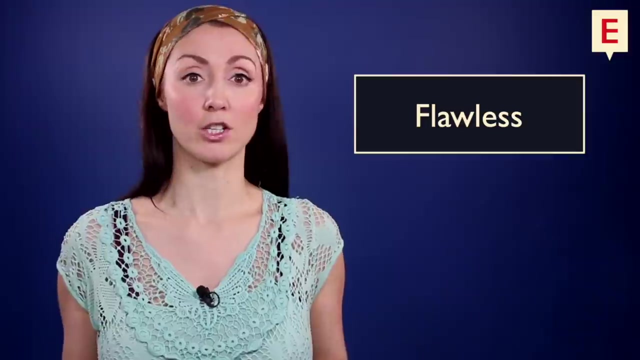 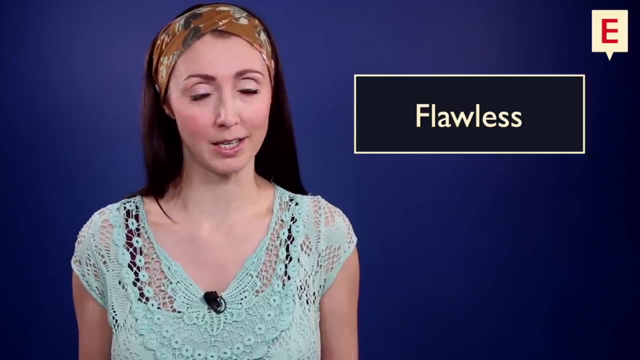 Excruciating. If something is excruciating then it is intensely painful. Having a broken leg can be excruciating. Number 40.. Instead of very perfect, try flawless Again. perfect is actually a non-gradable adjective, although you still might hear it used with the word very from time to time, even though it's grammatically incorrect. 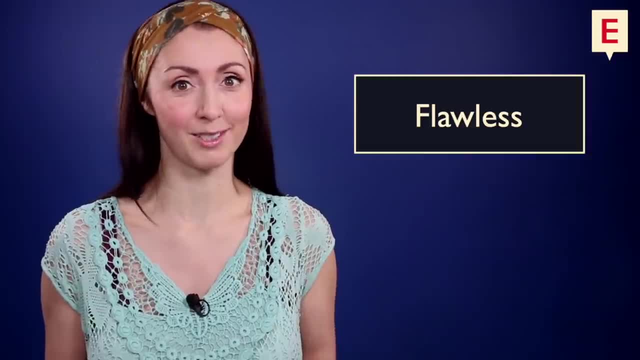 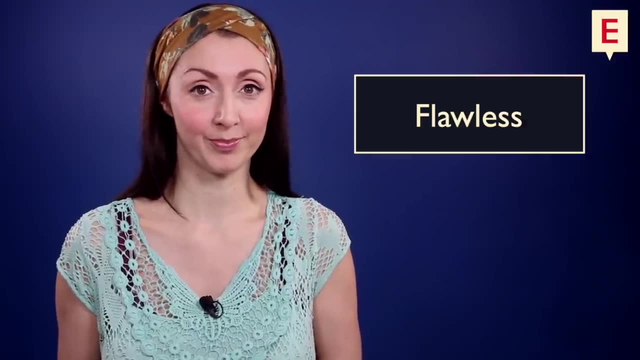 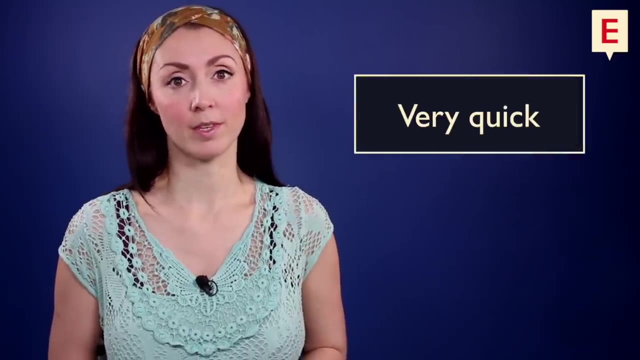 Using a different, more unusual word like flawless helps you to stand out. So if something is flawless, it means it's without flaws or imperfection. She gave a flawless answer and got a perfect score, Number 41.. Instead of very quick, try rapid. 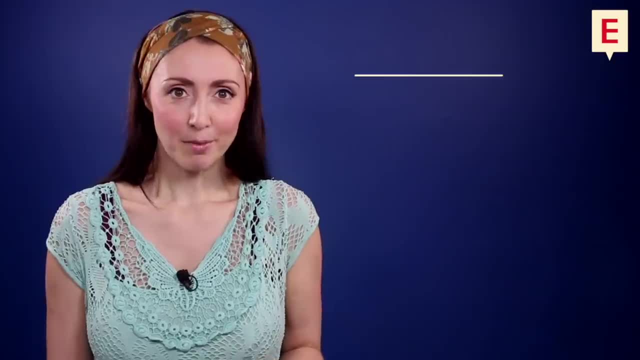 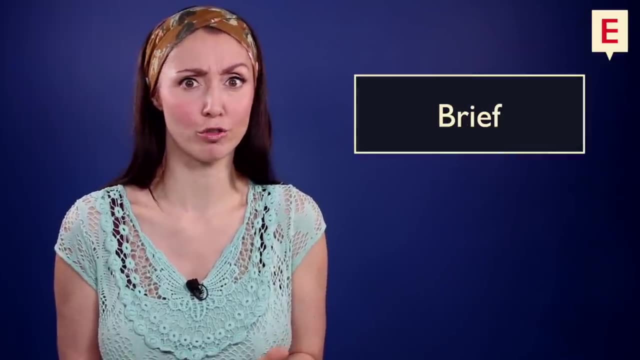 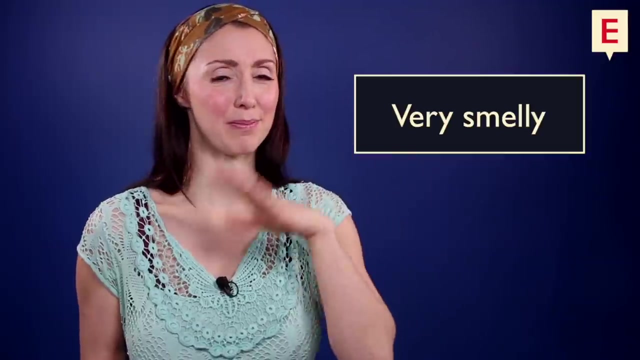 I got a rapid response to my email. Number 42.. Instead of very short, try brief. If something is brief, then it's of a very short duration. We had a brief catch up. Number 43.. Instead of very smelly, try pungent. 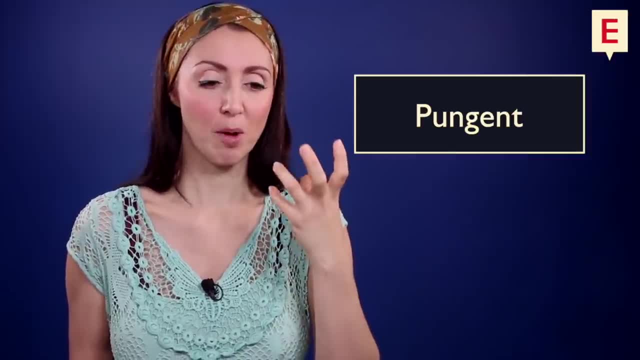 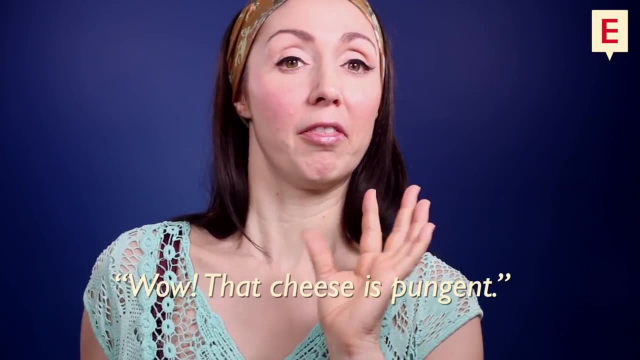 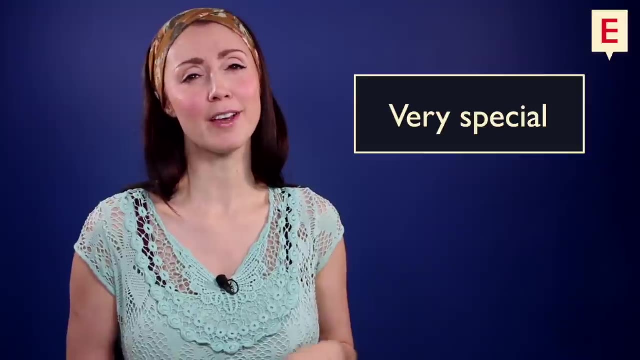 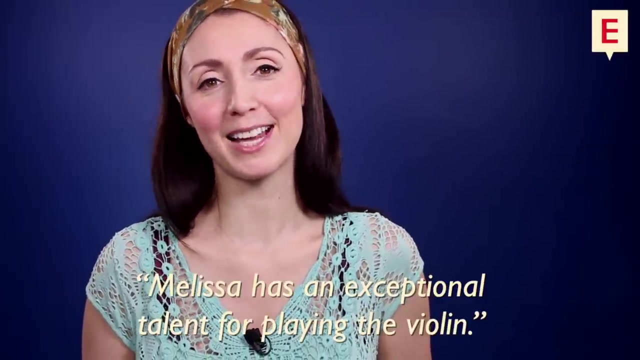 If something is pungent then it has a sharply strong taste or smell- Oh, usually unpleasant. Wow, that cheese is pungent. Number 44. Instead of very special, try exceptional. Melissa has an exceptional taste, An exceptional talent for playing the violin. 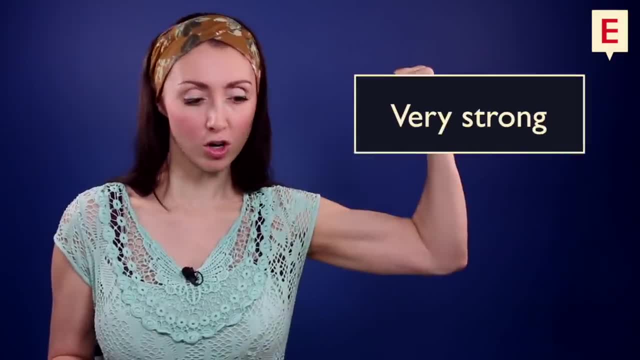 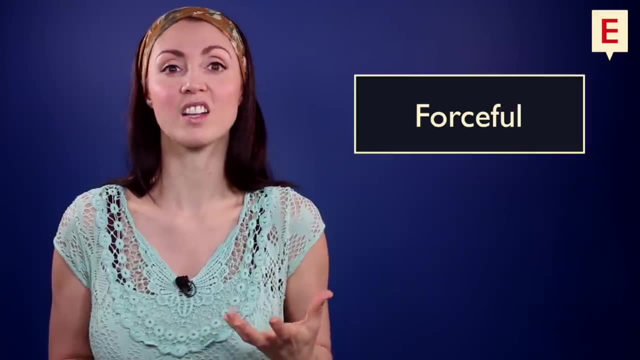 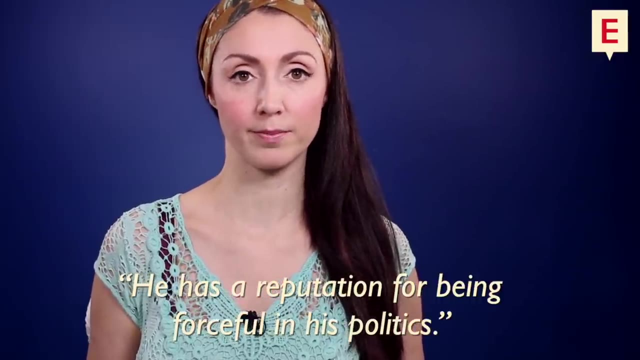 Number 45.. Instead of very strong, try forceful. If someone or something is forceful, then they are strong, assertive, vigorous and powerful. He has a reputation for being forceful in his politics. Number 46.. Instead of very stupid, try idiotic. 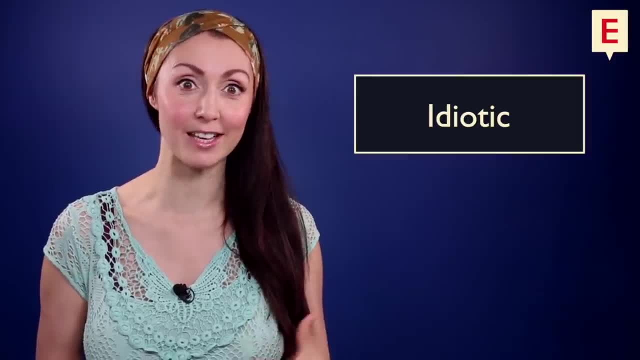 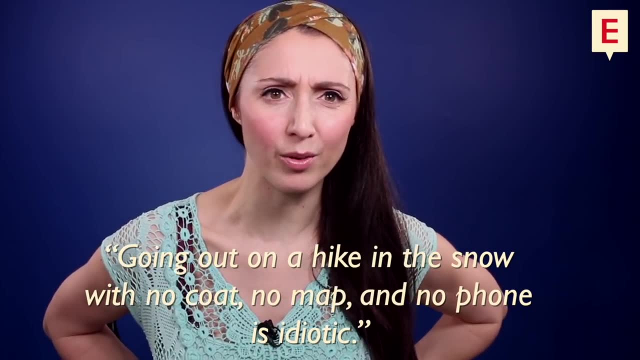 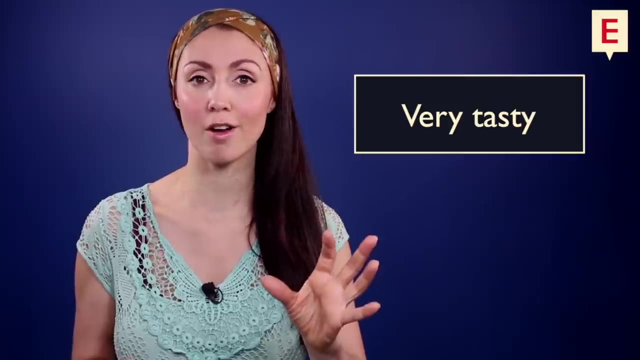 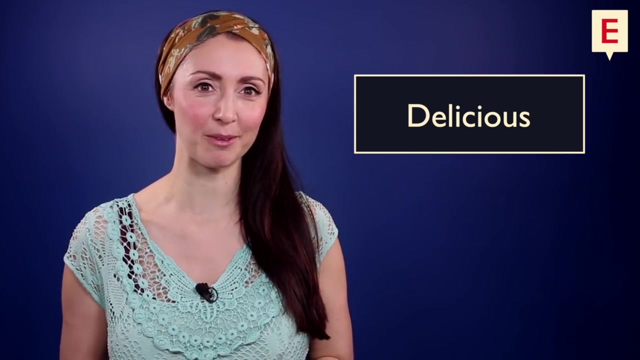 Now the dictionary definition of idiotic is literally very stupid. Going out on a hike in the snow with no coat, no map and no phone is idiotic. Number 47. Instead of very tasty, try delicious. If something is delicious, then it is extremely pleasant to eat. 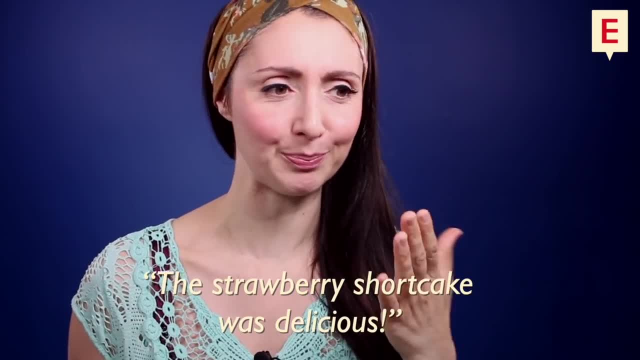 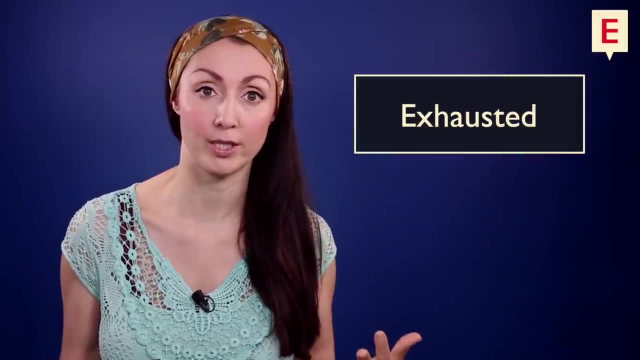 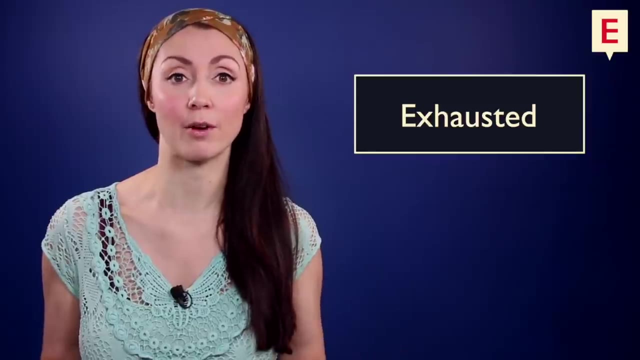 The strawberry shortcake was delicious, Mmm. Number 48.. Instead of very tired, try exhausted. If something is exhausted, then it is completely used up, Like if a battery runs out, it is exhausted. We also use this word to speak about people who are incredibly tired.